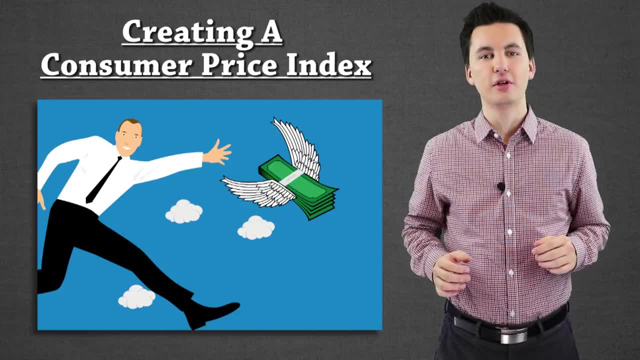 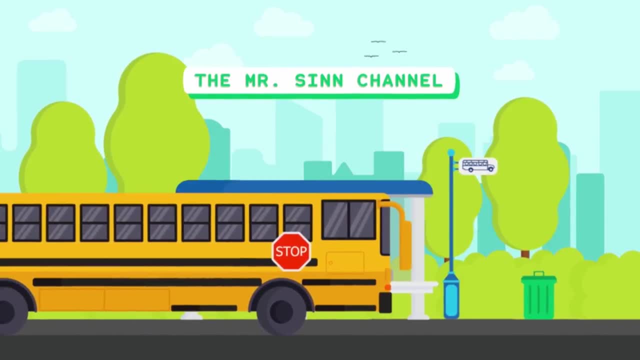 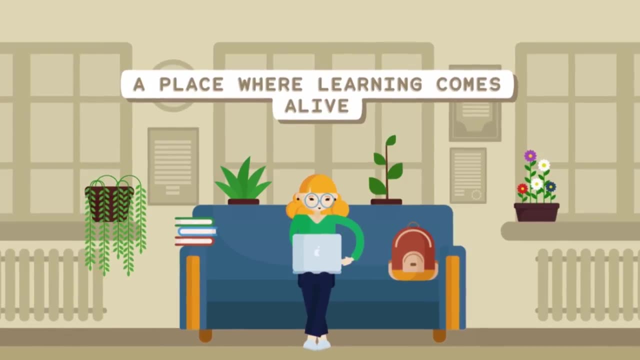 Hey there, Econ students. In this video we'll be looking at how to create a CPI, a Consumer Price Index, and also how to find inflation. So while watching this video, make sure to use the guided notes. You can find the guided notes. 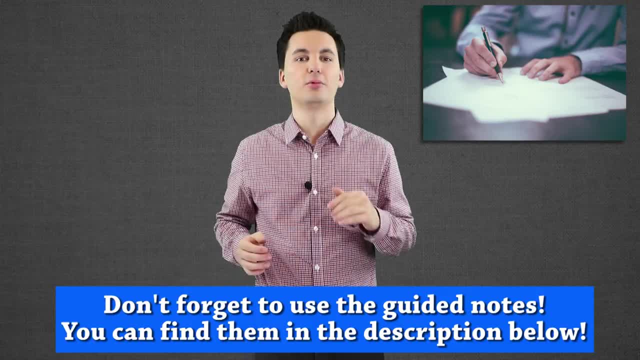 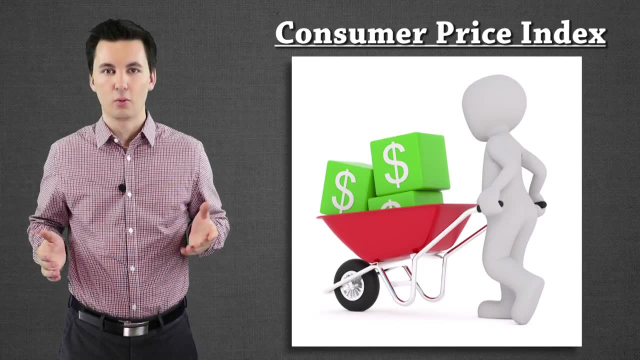 in the description below. The guided notes go along with the video and will help you understand the content better. So let's just start talking about CPI, a Consumer Price Index. We're going to cover this first and then we'll get into inflation. Now, a Consumer Price Index is used to kind of see. 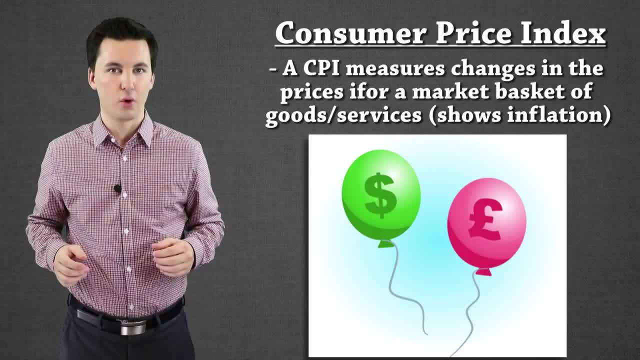 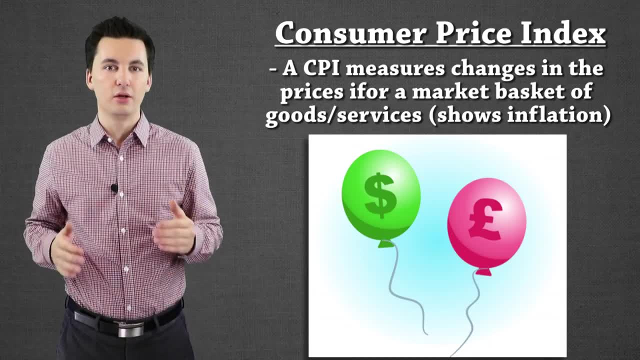 what's happening with inflation. Now, we're going to have to have a base year for this. When we're looking at inflation, we have to understand that the value of money changes over time, And when we have inflation, that means our purchasing power is going down. So a Consumer Price Index is used. 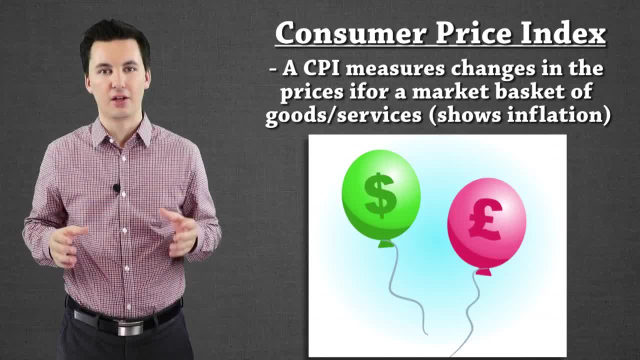 to kind of see what's happening with inflation. And when we have inflation that means our purchasing power is going down. So a Consumer Price Index is used to kind of see what's happening with inflation. What's going on with inflation with a certain basket of goods? Normally we'll have the same. 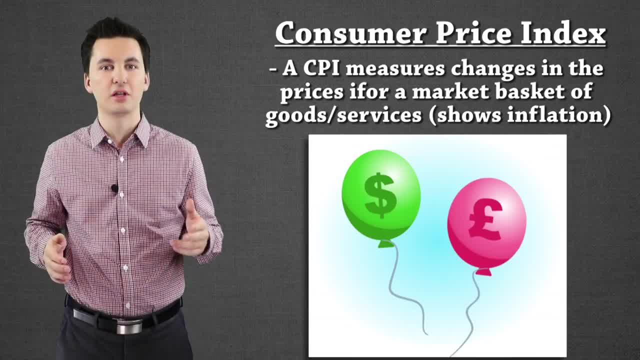 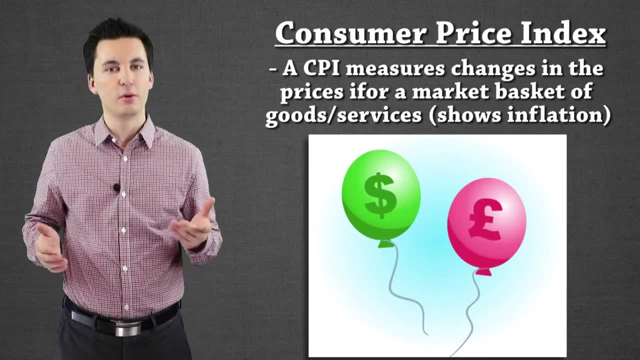 goods compared in a CPI every single year, So that way we can see how the value of those goods has changed. If those goods cost more, we've seen inflation. If they've cost less, then we might see deflation occurring. To calculate this out, we first have to create a CPI. First thing we'll 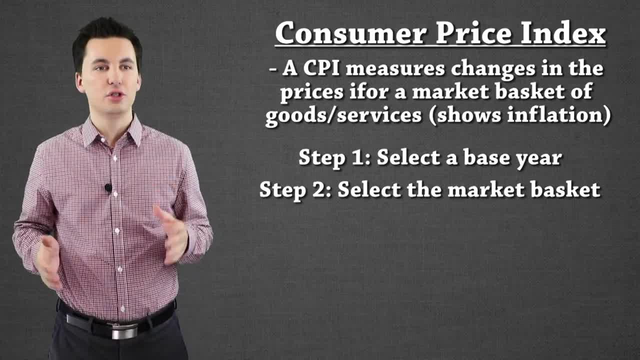 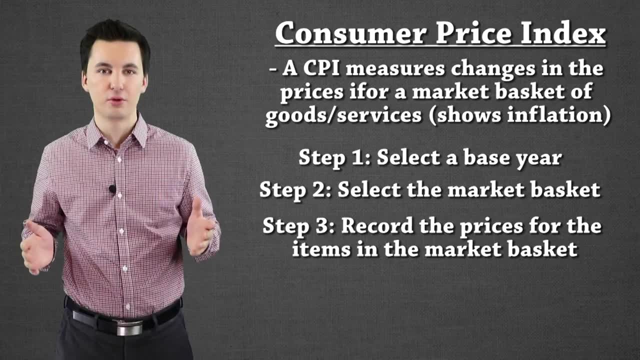 have to do is select a base year. That's step one. Step two is we'll need to actually select what's going to be in our basket, So we're going to have to select a base year. That's step one of goods. Step three: we'll record all of the different prices for each of our years and then 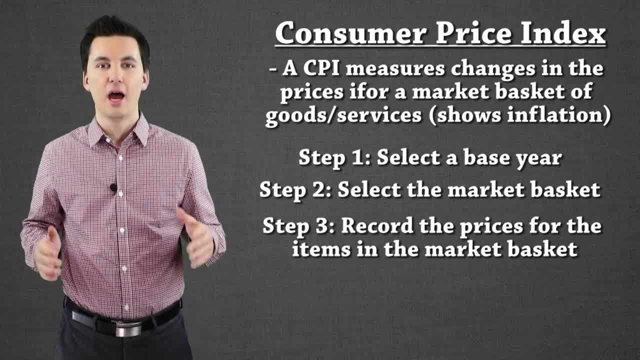 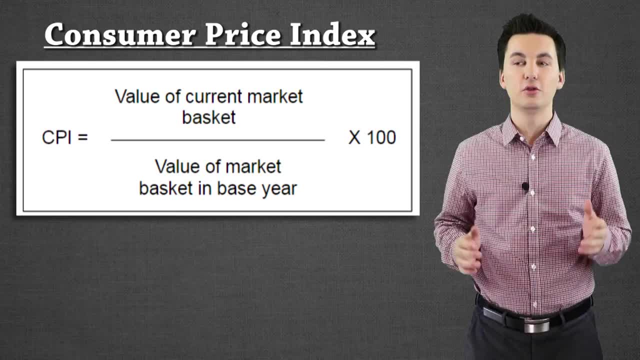 we'll times that by the quantity, So we'll be able to see exactly how much our basket costs. Step four is the math part. Now, before you freak out about math, it isn't that bad. We're going to use this formula: Our CPI will equal the current value of our market basket, So this is referencing whatever. 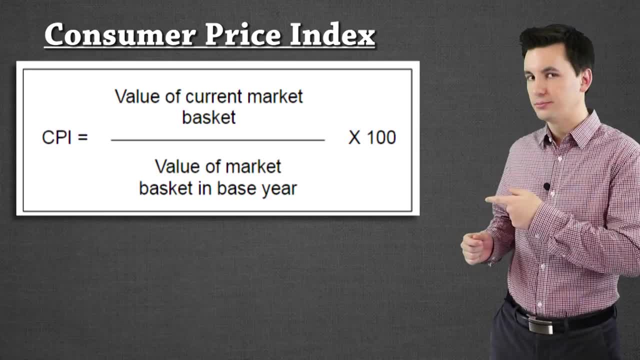 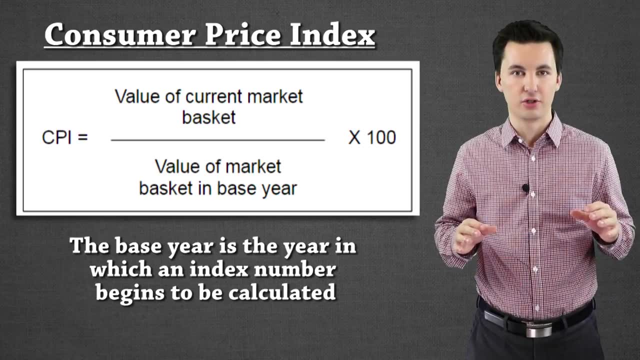 year we're trying to find and then we're going to divide it by the base year. Now, I've already referenced the base year, but a base year is going to be the year that we're going to use that value. This value, whatever our base year is that we decide to pick, that is going to then be the value that. 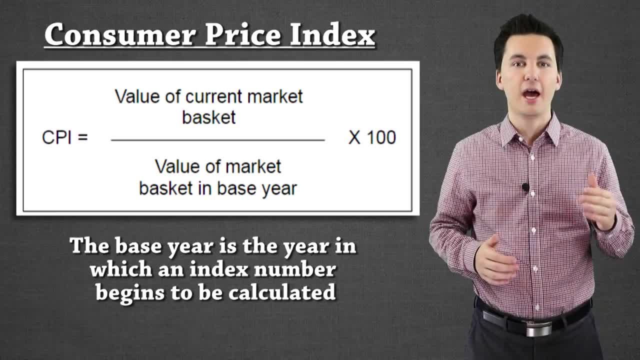 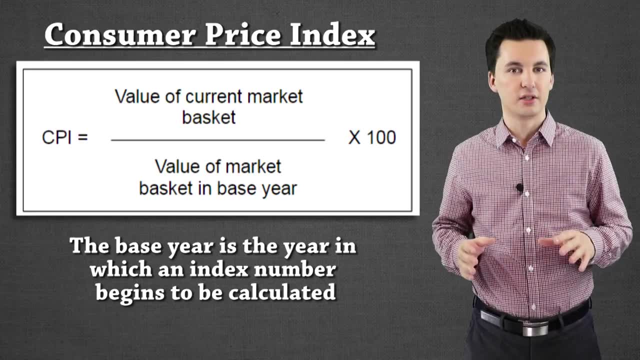 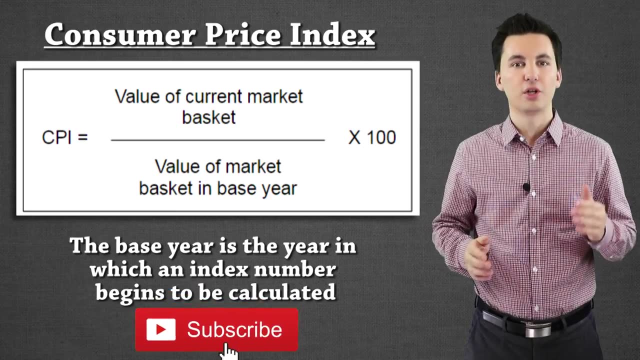 we'll compare of our money to all the other years. After dividing, we times it by a hundred and this is going to get our CPI. Now, this isn't necessarily a percent, it's an index number, but it does show us a percent change compared to just the base year- Not between year to year, but it shows what's. 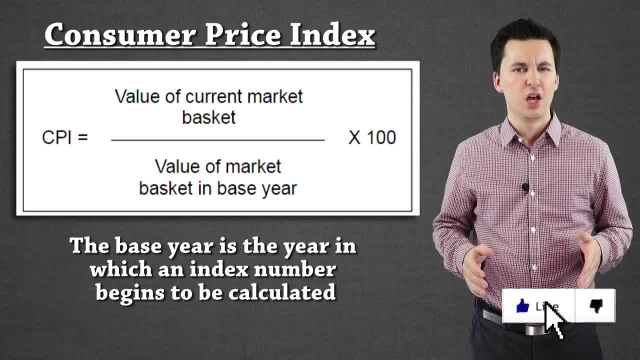 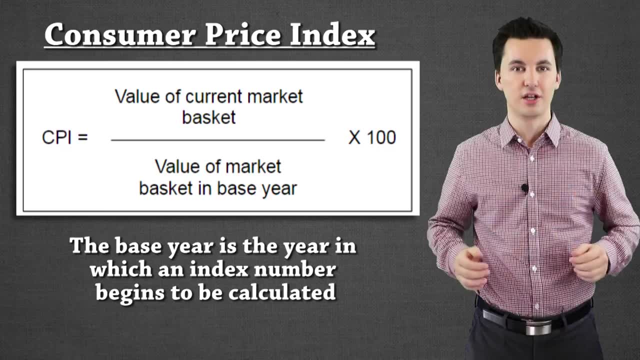 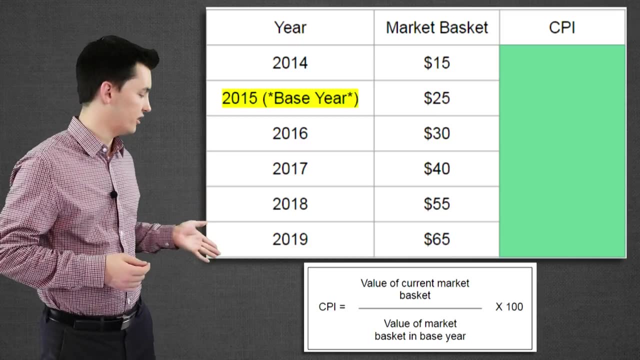 happened with the value of money In comparison to our base year. So let's actually look at this in practice and kind of see what we're talking about. It's easier to visualize it when we're actually seeing the numbers firsthand. So over here right now you can see I have a couple different years. I've 2014, all the way to 2019.. 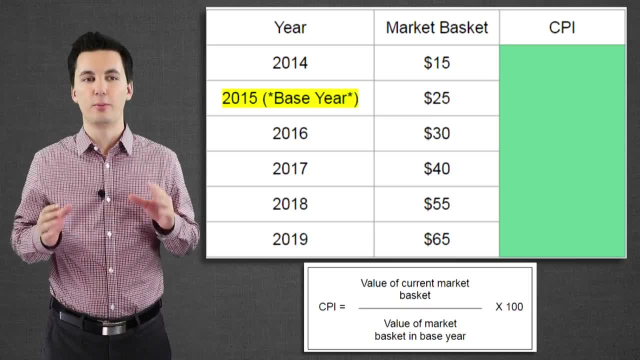 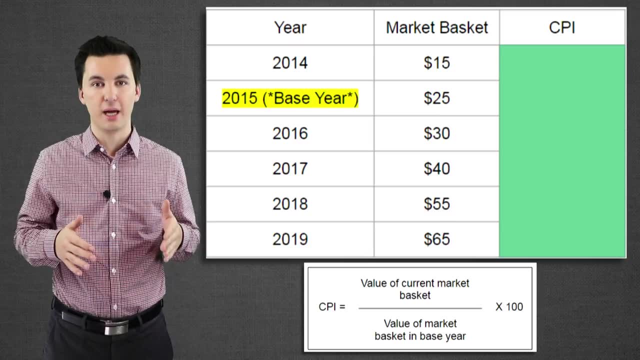 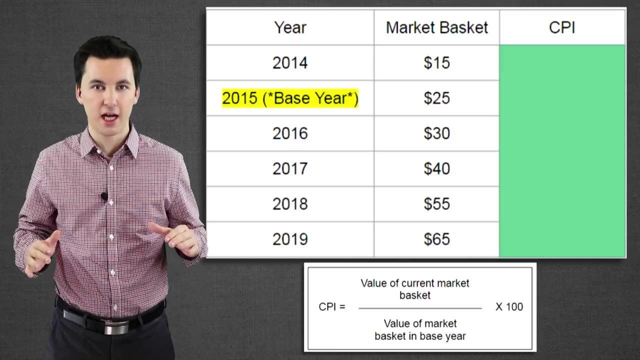 Now, one of the important things to realize here is we've selected this base year at 2015.. Now, what this means is: this is the year I'm going to use to compare that value of the basket to everything else. I'm going to note: the CPI for the base year will always be a hundred. Every single time, the base year will be a hundred. 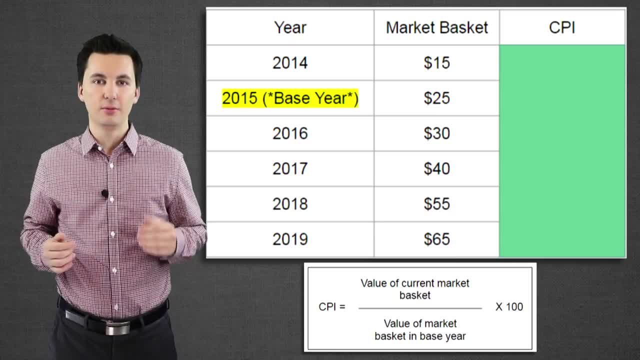 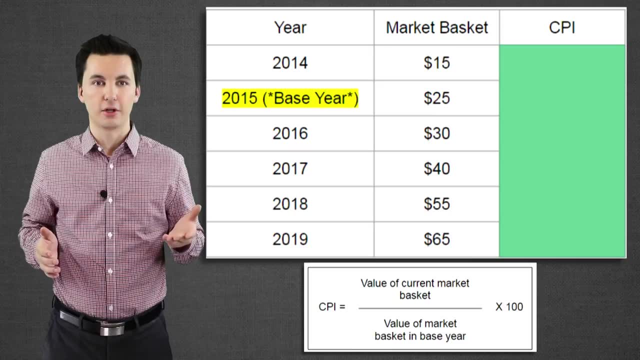 Remember that. And the reason why is: if I'm looking at the value, if I'm trying to calculate out what's happening with our CPI, I'm going to use the formula we talked about earlier. I'm going to take the current value of the market basket and divide it by the base year. 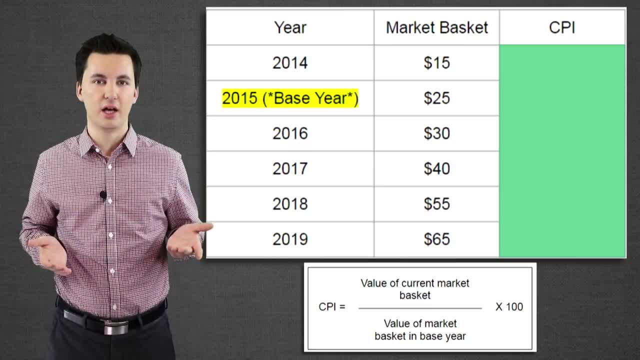 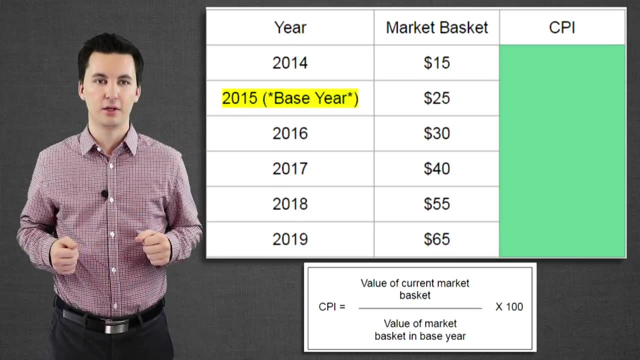 Well, if I'm talking about the base year, I'm dividing the same thing by itself. So for here I'd be taking 25 divided by 25.. That's going to give me one, And then I would times it by a hundred. So my base year is a hundred to CPI a hundred. 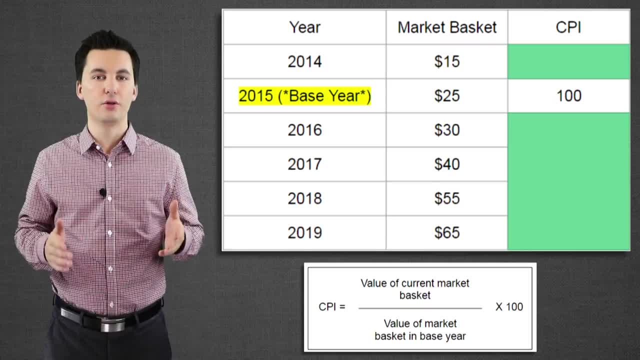 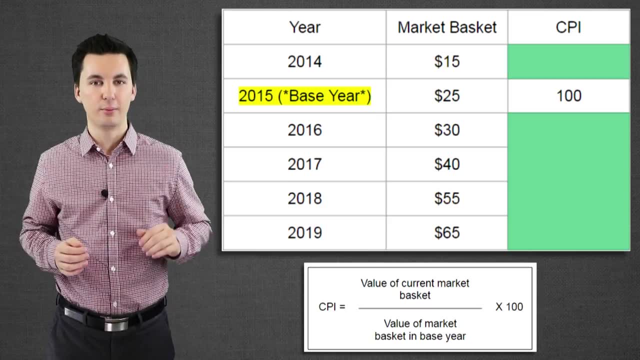 Now try to figure out what the CPI would be for all the other years. Remember the formula. The formula is our current market basket, Whatever year we're trying to find, divided by the base year market basket and times that by a hundred. Pause this video and try to figure it out. 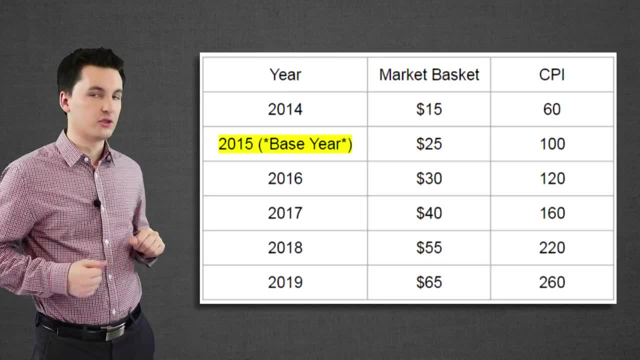 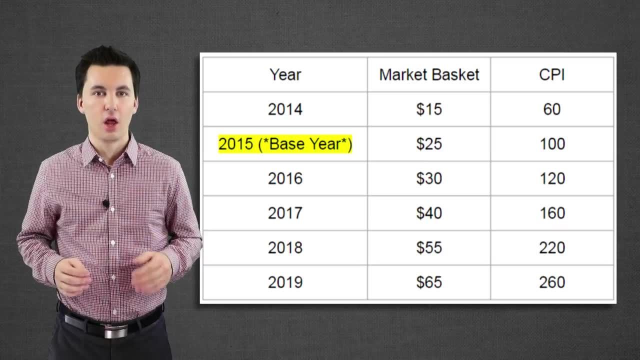 Did you get it? Check your answers. right now You can see the answers on the screen. One of the things to note is, when we're looking at this, we're not seeing inflation rate between every single year. we're seeing it in comparison to our base year. so for 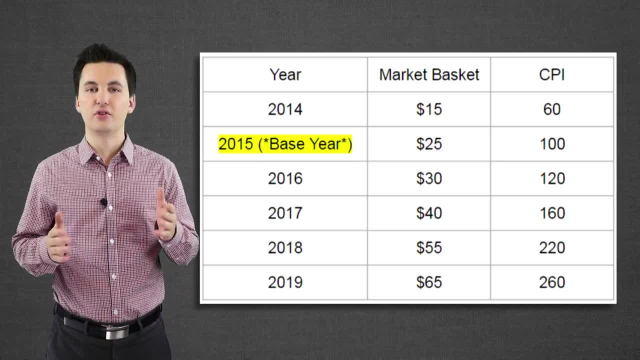 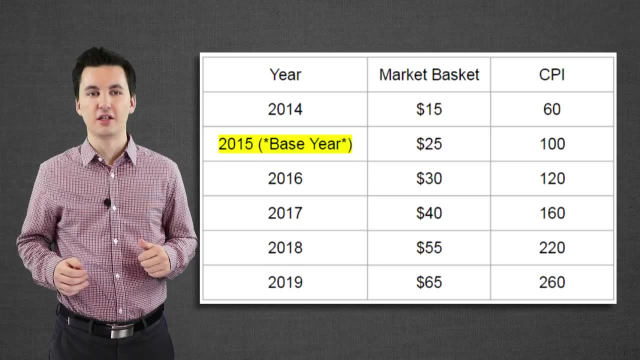 example, if i'm looking at 2016, i have a cpi of 120.. that means i've had 20 inflation since my base year. if i look at 2017, i can see it's 160.. this means that i've had a 60 inflation rate from. 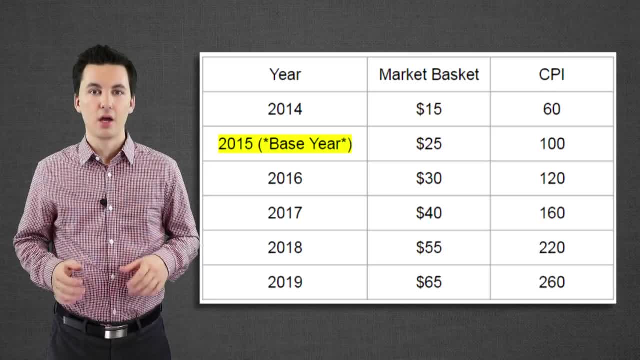 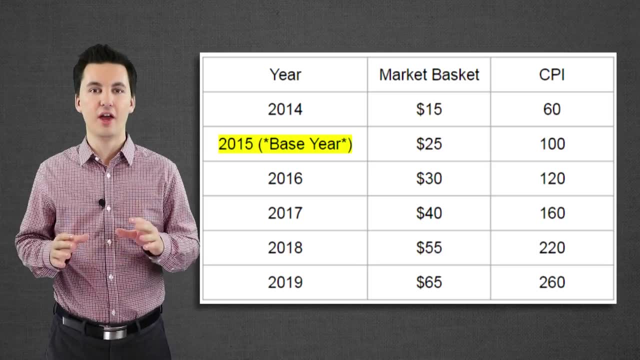 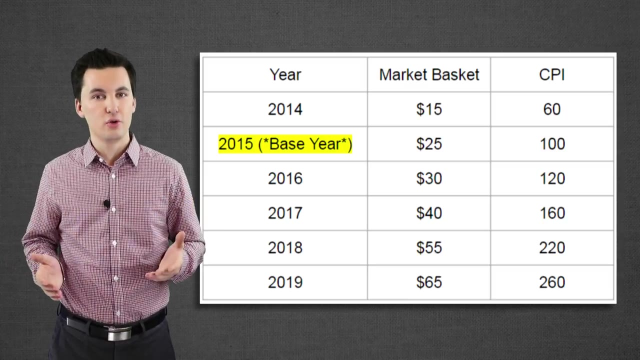 the base year, not from 2016.. the next thing we're going to go into is actually how to find an inflation rate between years. this is again just showing us what's happening between the base year with inflation. hopefully, the cpi is making sense how to find it. it isn't too bad, it's just. 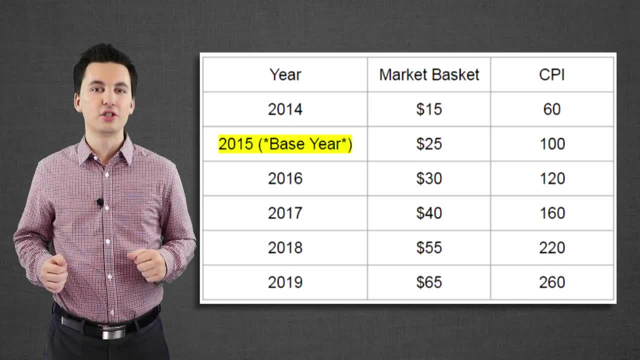 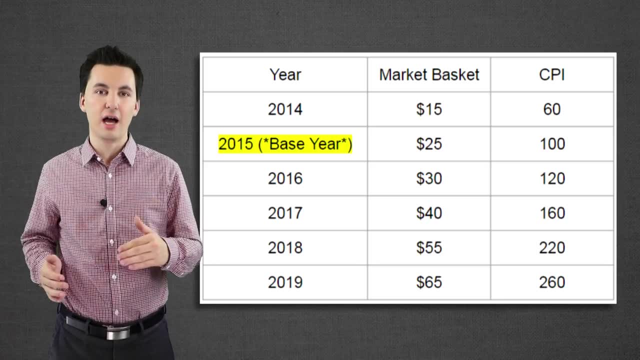 important to understand the formula and what's going on. one other thing to note is: if we're ever going below 100 now, like we can see for 2014, we're actually seeing deflation. our value is going the opposite way. instead of inflation occurring, where we're losing purchasing power, we're actually 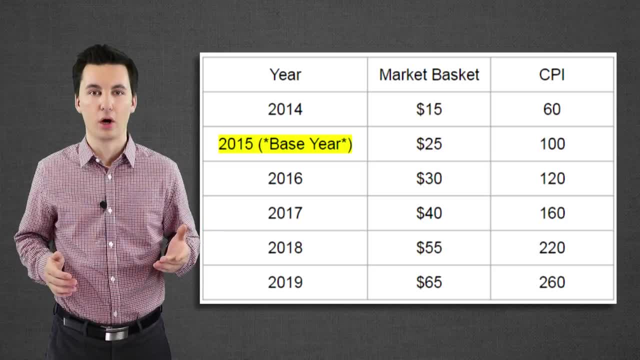 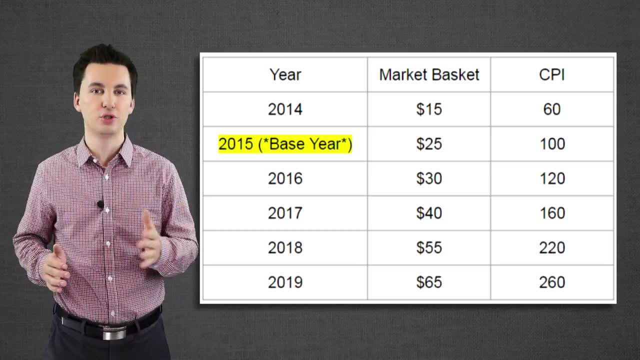 seeing it where we're gaining money, and we're actually seeing it where we're gaining money purchasing power. our money is worth a little bit more. so that's something to consider. now let's go on to the next thing, where we'll actually look at how to find the inflation rate between two years. 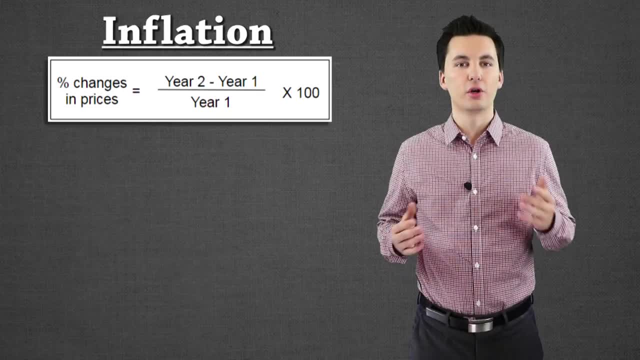 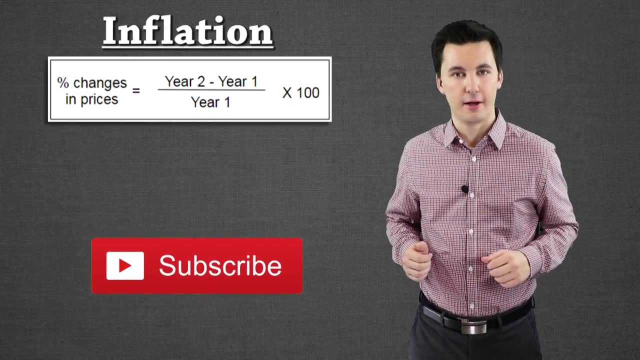 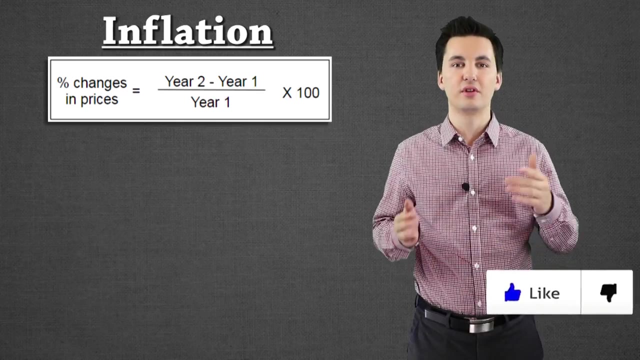 so when calculating out the inflation rate between two years, we're going to use the following formula: we're going to have our year two minus year one divided by year one, times it by a hundred. that's it now. this is important to understand. when looking at a problem, you have to have the previous year. 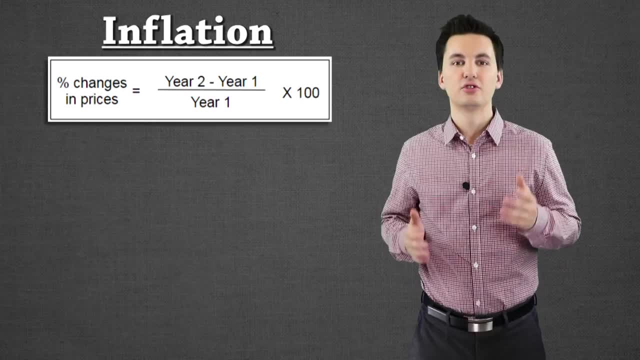 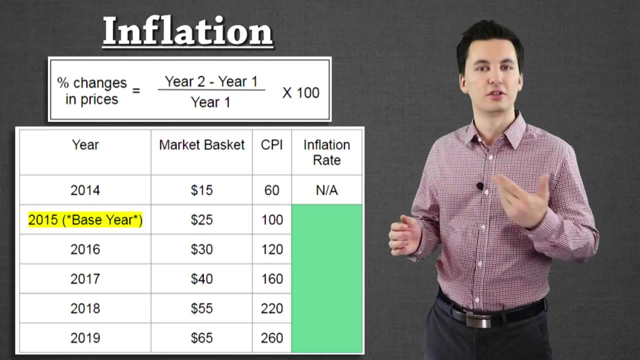 to be able to find the inflation rate between two years. so let's take a second and look back at the data that we just calculated out for our cpi. you can see here we have again 2014 to 2019.. one of the things to note. 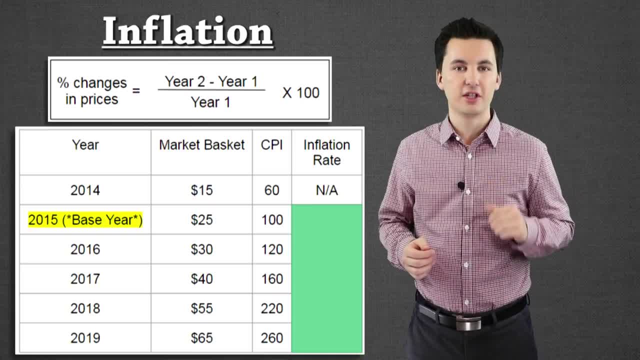 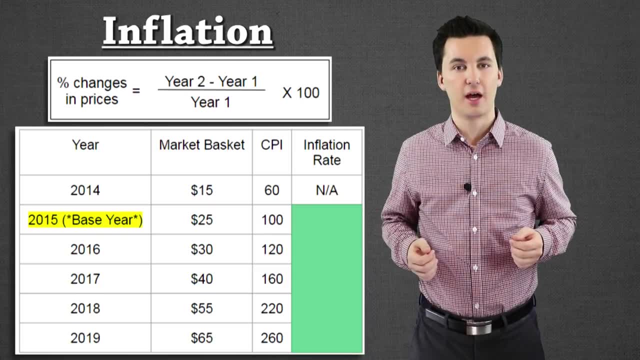 here if we want to find the inflation rate between years. we actually can't for 2014.. the reason why is we don't have the data for 2013.. so we wouldn't be able to solve that. however, let's go and do one. 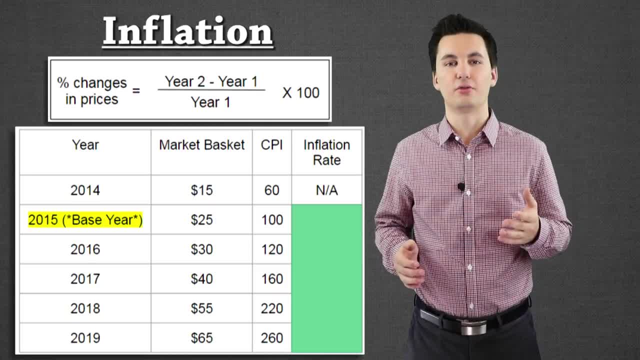 together and then we'll see if you can figure out the rest of the table. let's calculate out the inflation rate for 2015.. let's go and do one together and then we'll see if we can figure out the rest of the table. let's calculate out the inflation rate for 2015.. 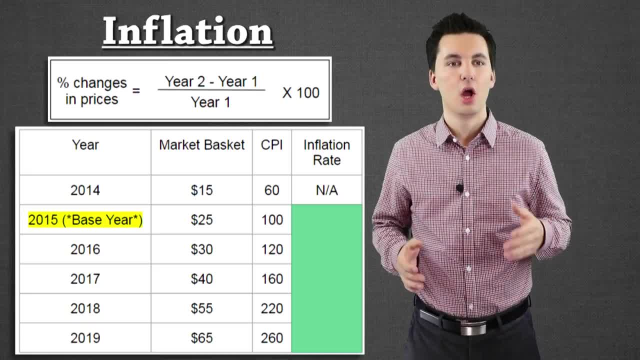 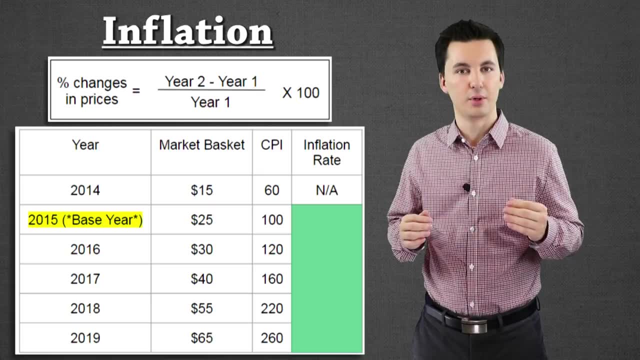 so we're looking from 2014 to 2015.. what we're going to do here is take our hundred, which is going to be our year two. that's the current year. we're trying to figure out what happened. we're going to minus it by the 60, because that's our cpi for year one. then we'll divide it by 60.. we're. 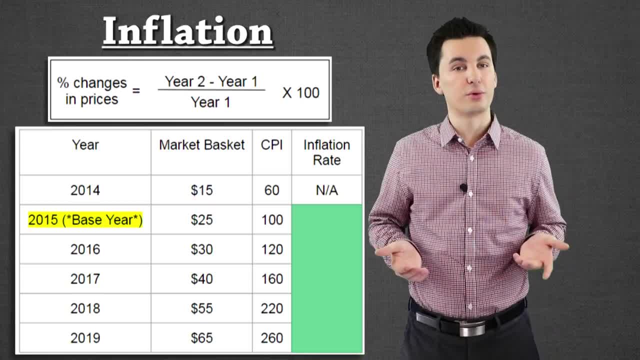 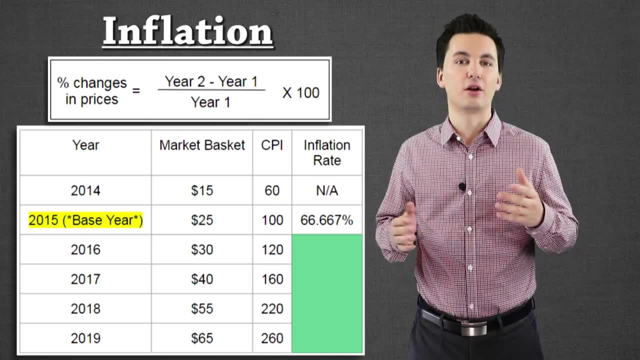 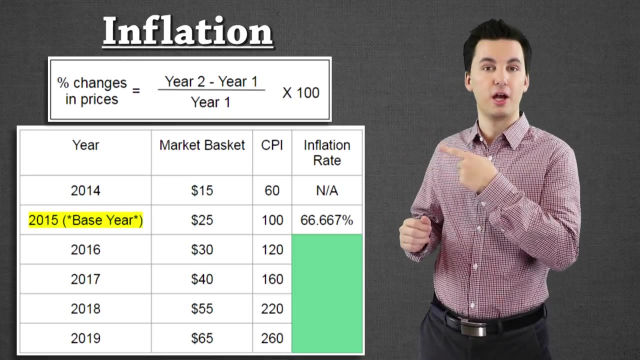 then going to times our answer by a hundred, which will turn it into a percent, so we're going to have 66.6667. it's kind of repeating percent. that would be our inflation rate between these two years. is it making sense? try to figure out the rest of the table. i'll leave the formula up there, but use